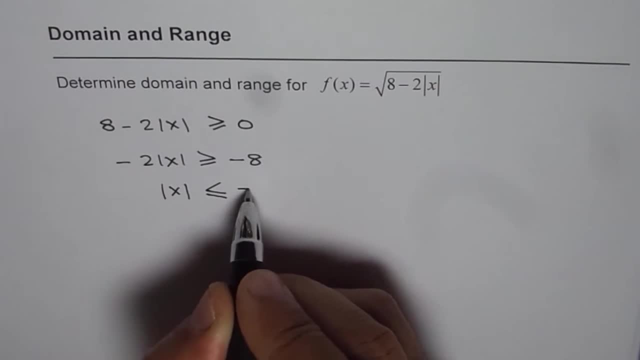 changes. So it becomes less than equal to minus 8 divided by minus 2.. That means absolute x is greater than equal to 0.. x should be less than equal to 4.. If absolute value of x is less than equal to 4, it really. 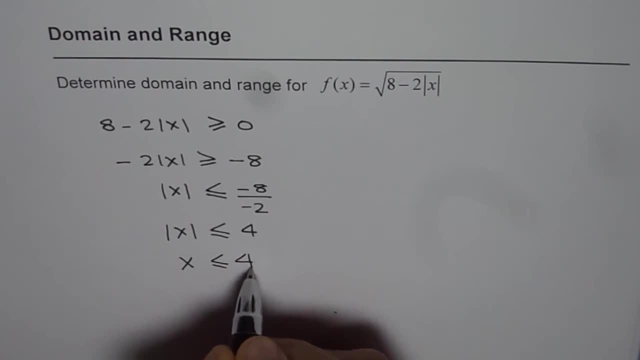 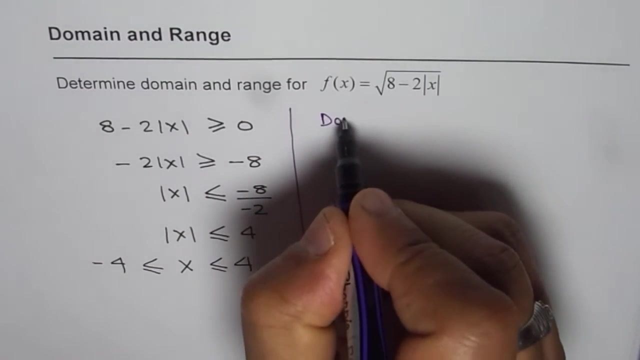 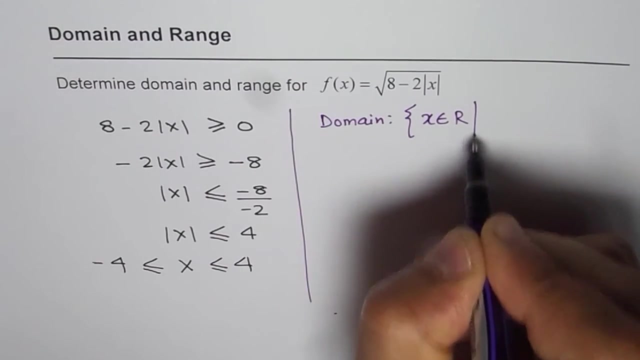 means that x is less than equal to 4, but greater than equal to minus 4.. So that is how we solve inequality. So solving this inequality we get: x is between minus 4 and plus 4.. So that is the domain for the given function. right, So we can write domain as x belongs to real numbers, so that 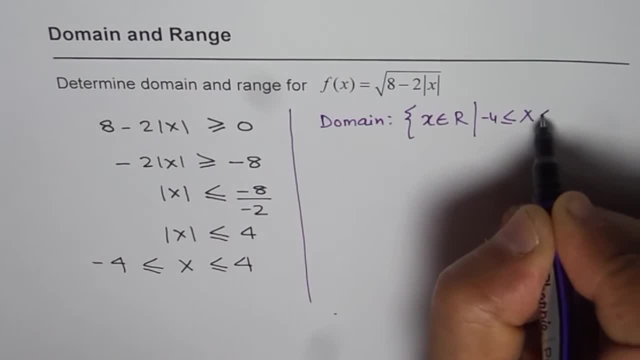 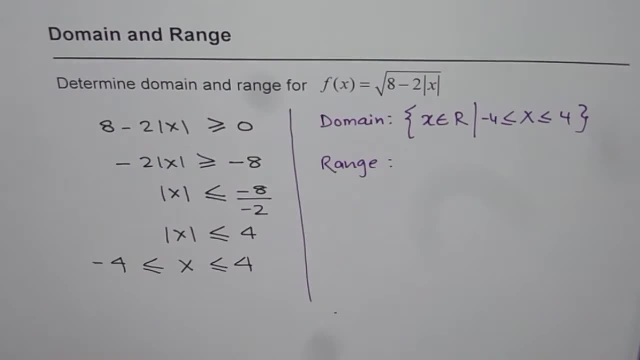 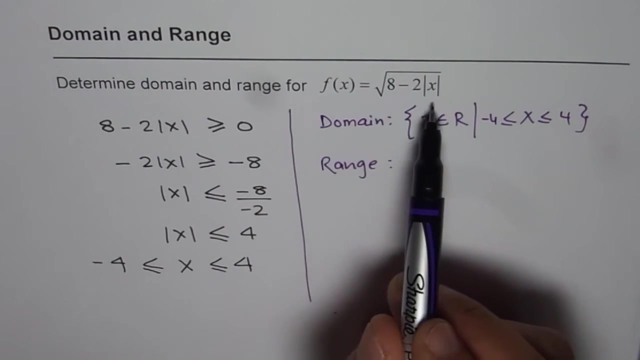 x is greater than equal to minus 4 and is less than equal to plus 4.. Now, how about range? Range is going to be positive. Now the maximum value will be when absolute x is 0.. 8 minus something positive will be maximum when x value. 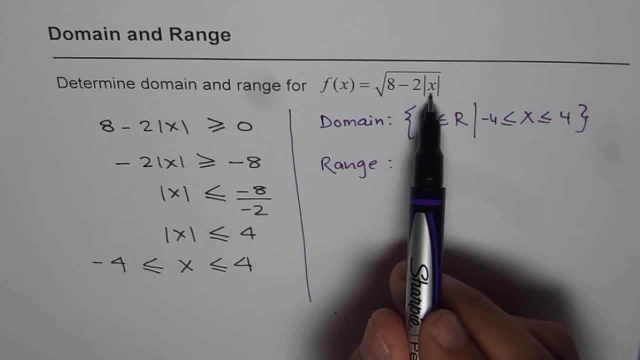 is 0,. right, You are taking away minimum. If x value is 0, then we get absolute x as 0. So we get square root of 8 minus 0.. To find range, what we can do is we can substitute these values to find. 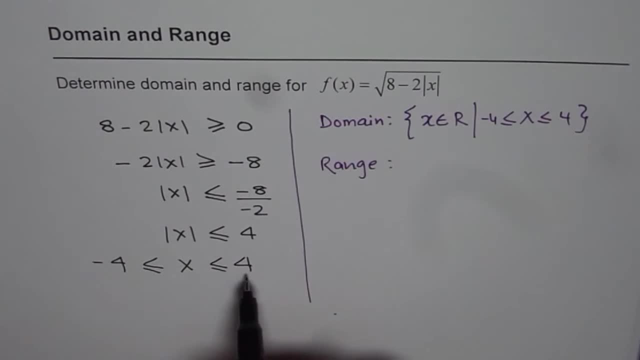 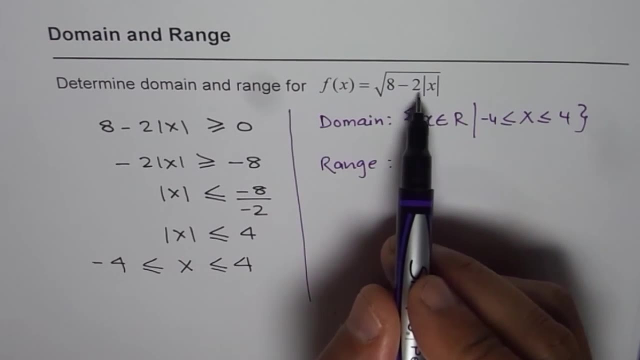 the extreme values, which are: if I write minus 4 or minus 4,, then we can substitute these values. If I write minus 4 or 4,, we get 8 minus 2 times 4, which is 0, right, So the range, basically, you can. 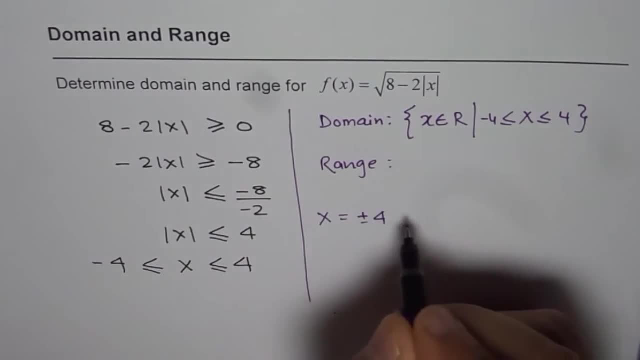 substitute: x equals to plus minus 4, and then find what is the value of f of x. f of x is square root of 8 minus 2, times plus or minus 4, either one of them. It will be positive. So this value is equal. 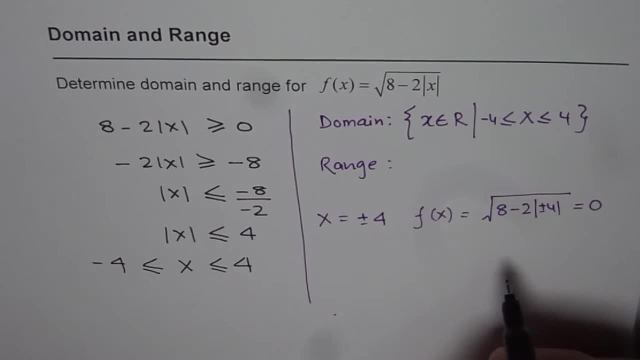 to 0.. So that is the minimum value of x. So that is the minimum value of x. So that is the minimum value for the range. To get the maximum value we can substitute 0 for x, right? So f of 0 is.